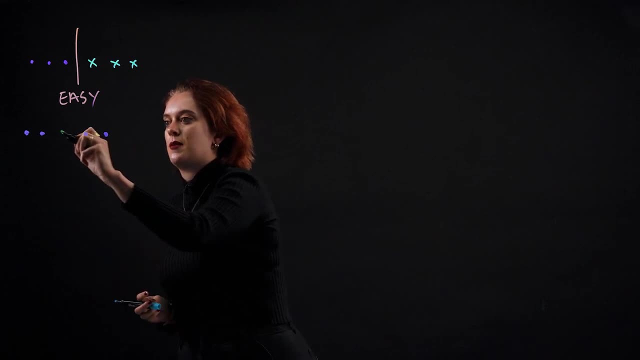 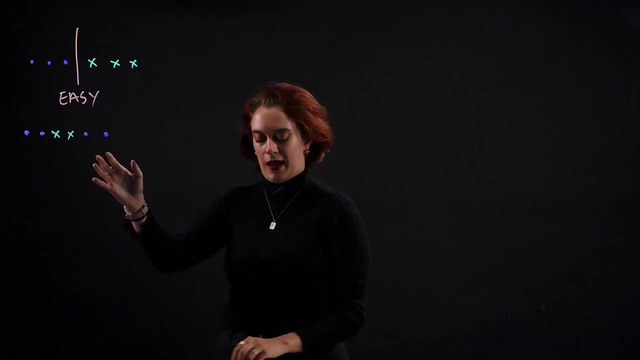 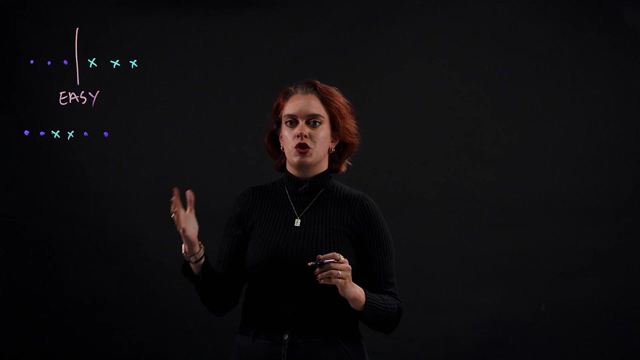 for example, if our data is arranged like this, perhaps with the crosses in the middle, now there isn't a single line that we can draw on this plane to classify the data into two discrete groups. so, in order to solve this problem and classify this data, what we need to do is we 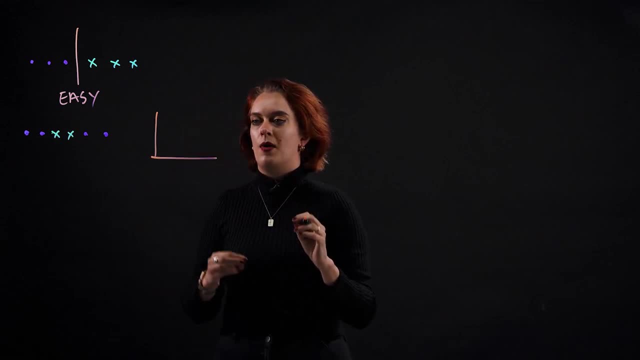 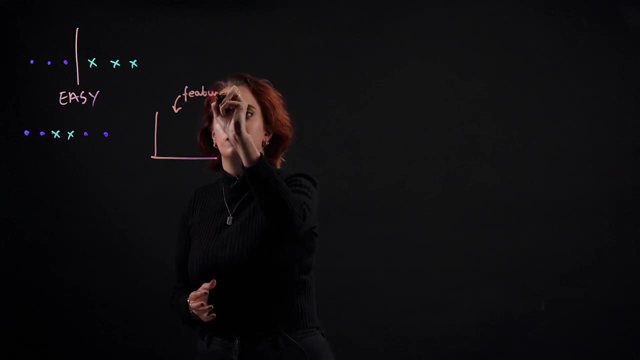 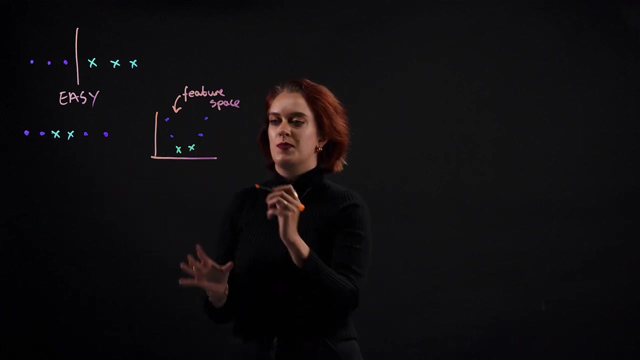 need to map this data into a higher dimensional space, which we're going to call a feature space. then if we've mapped the data, for example, like this, we can now see: because we've mapped this data into a higher dimensional space, there is now a much easier way to classify this. 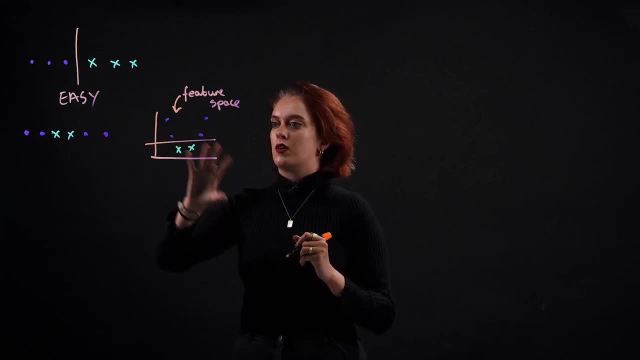 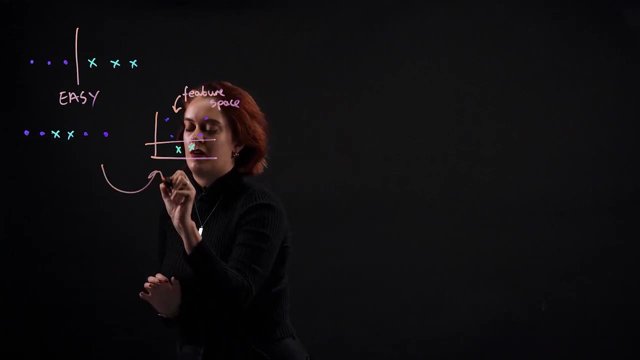 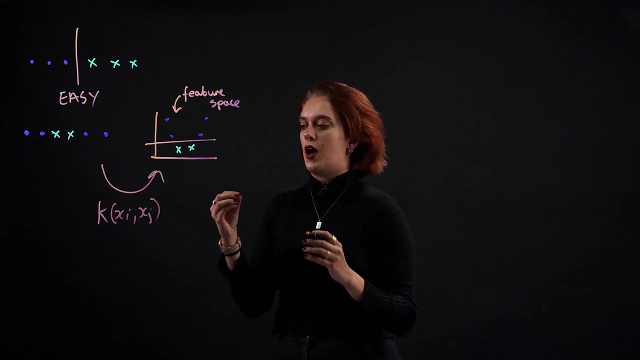 so how do we do this step of transferring our data, mapping it into a higher dimensional feature space? to do this, we can use kernel functions. kernel functions work by taking some underlying features of the original data set and using that to map those data points into this high dimensional feature space. 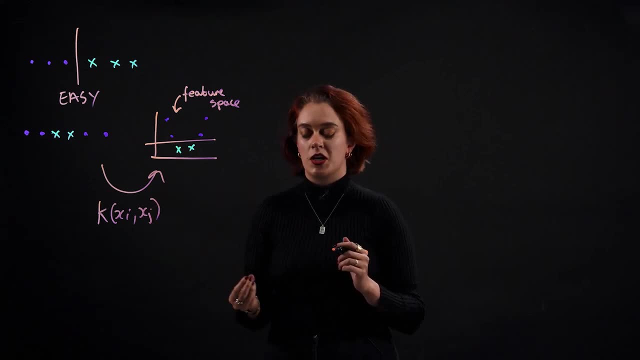 kernel functions are incredibly powerful and incredibly versatile, but they do face problems. sometimes they just give poor results and also the compute runtime can explode as the complexity of the data sets increase. if you're- if you're- an experienced machine learning developer, perhaps you've seen this already. if you're dealing with data that has very strong correlations, 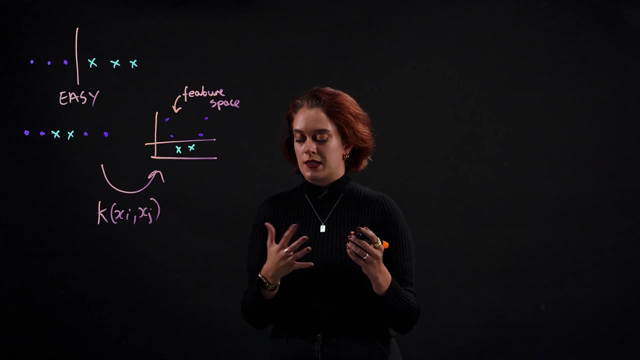 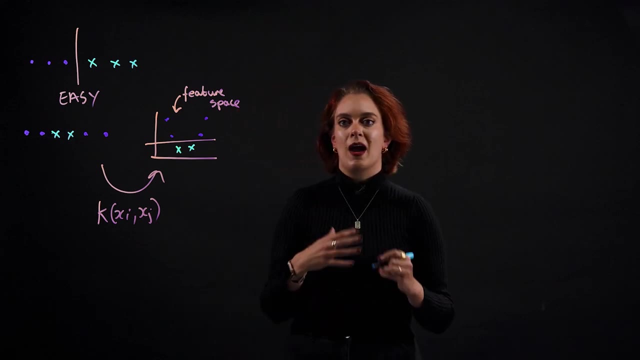 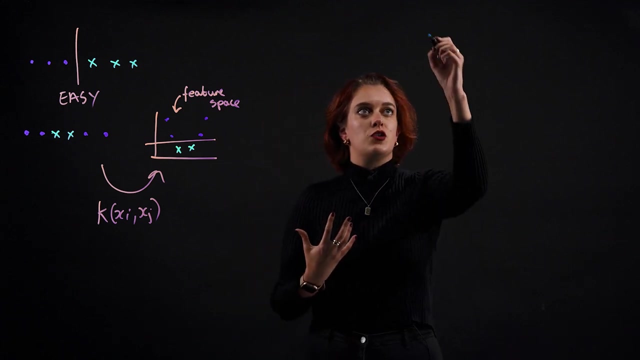 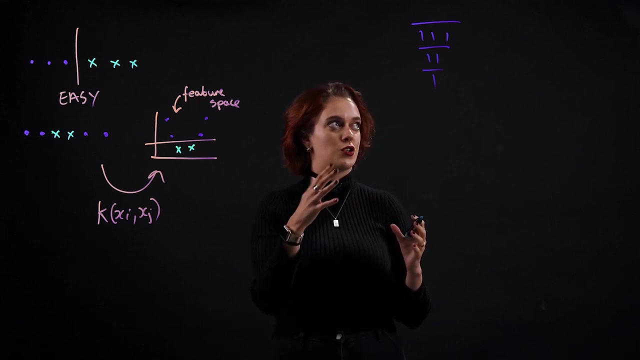 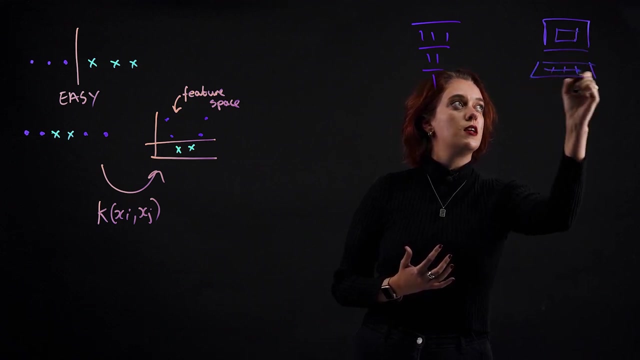 or perhaps if you're dealing with time series forecasting, where the data is very complex and at a high frequency. but quantum computers have the potential to provide an advantage in this space. they can be useful because quantum computers can access much more complex and higher dimensional feature spaces than their classical counterparts can, and they can do this because quantum computers. 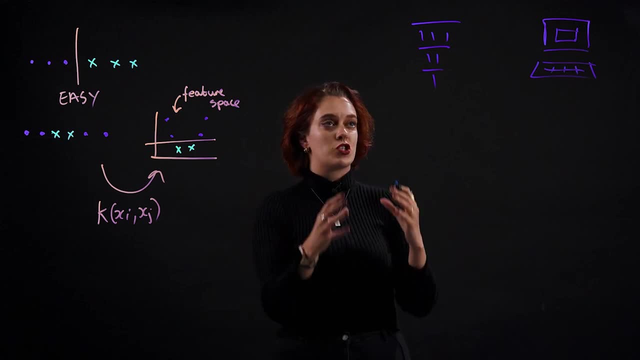 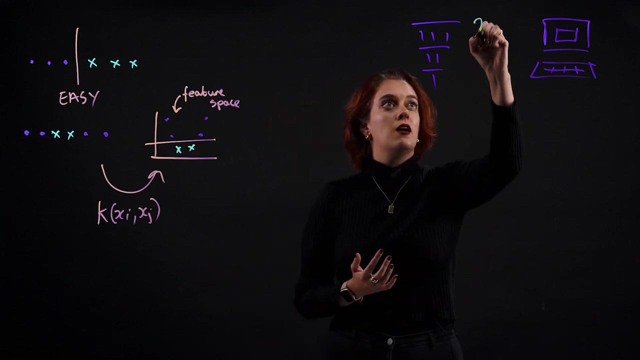 can. we can encode our data into quantum circuits, and the resulting kernel functions can be used to replicate on a classical machine. as well as this, those kind of functions also can perform better. in 2021, ibm researchers actually proved that quantum kernels can provide an exponential speed up. 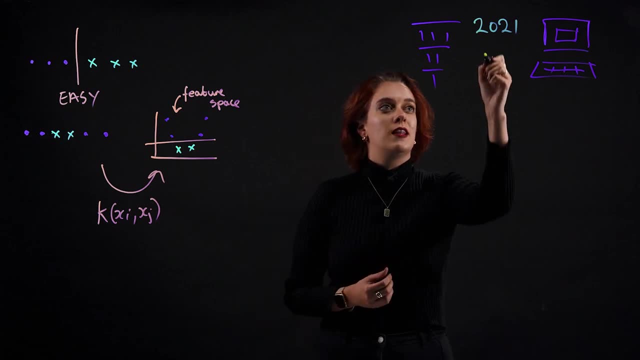 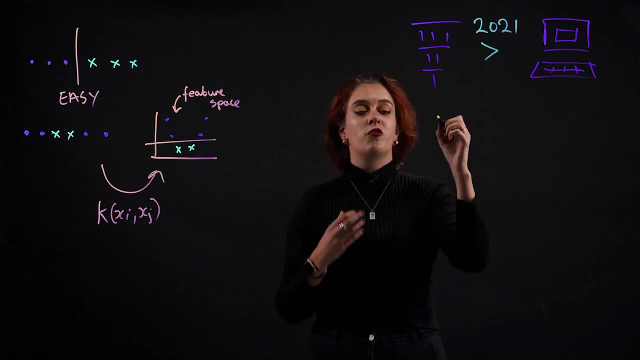 over their classical counterparts for certain classes of classification problems. so let's take a look at some of the things that we can do to replicate on a classical machine. so the first thing that we're going to do is we're going to do- is we're going to use quantum kernels to replicate on a classical machine. 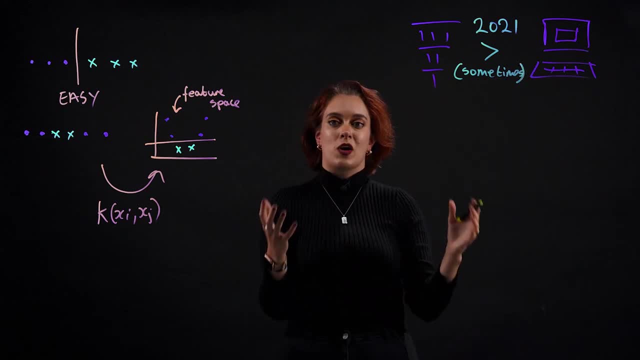 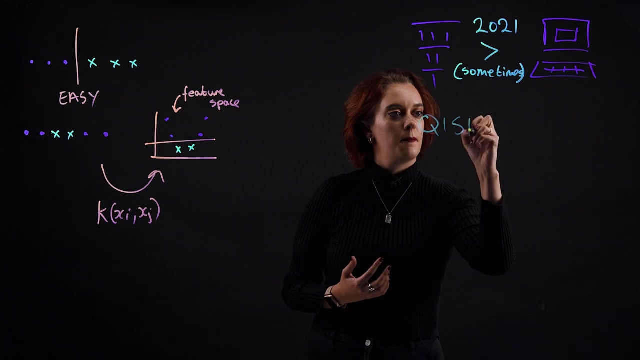 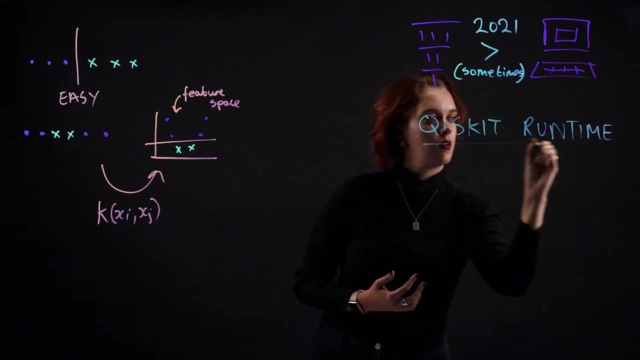 as well as this, there is a lot of research going into improving quantum kernels with structured data and kernel alignment. so, as you can see, this field is incredibly exciting. there's a lot of research going on in this space, and you can use qiskit runtime to easily build quantum machine learning algorithms with built-in tools such as the sampler primitive. 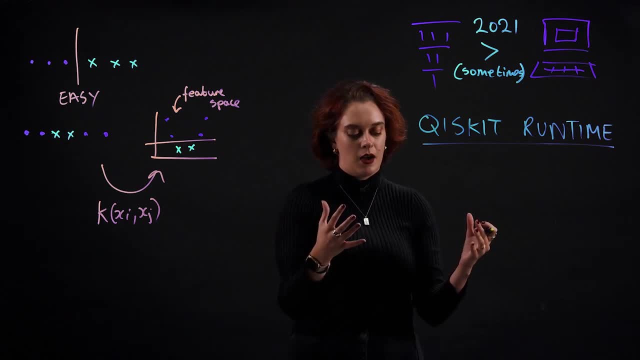 which primitives are unique to the ibm's qiskit runtime. these are essentially predefined programs that help us to optimize workflows and execute them efficiently on quantum systems. let's take, for example, our linear classification of quantum kernels, and we can use it to replicate on a classical machine. 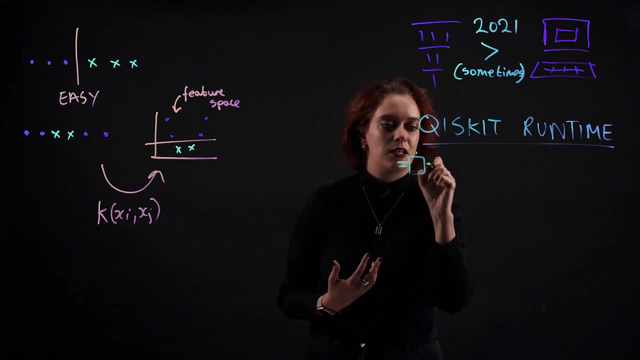 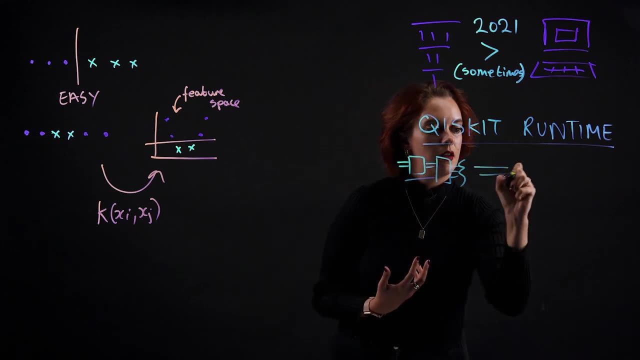 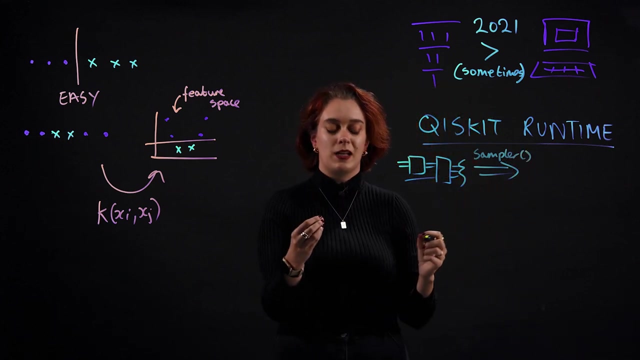 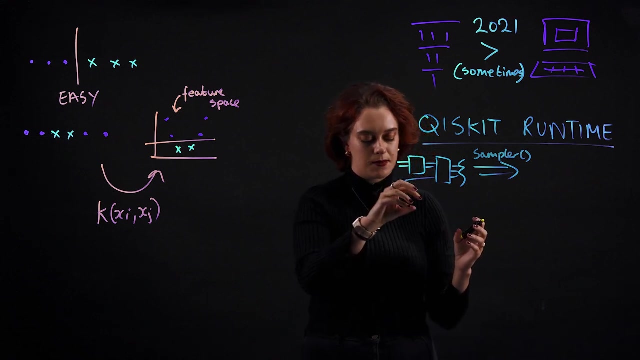 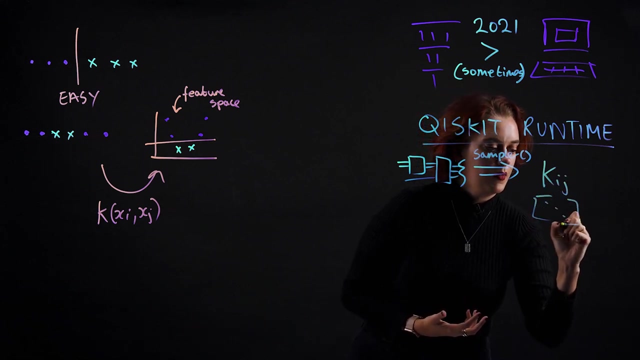 problem. let's say we have our data and we've encoded it into a quantum circuit. we can then use the sampler primitive to obtain quasi probabilities indicating the relationships between the the different data points, and these relationships can constitute our kernel matrix. and that kernel matrix can then be evaluated and used in even a classical support vector machine. 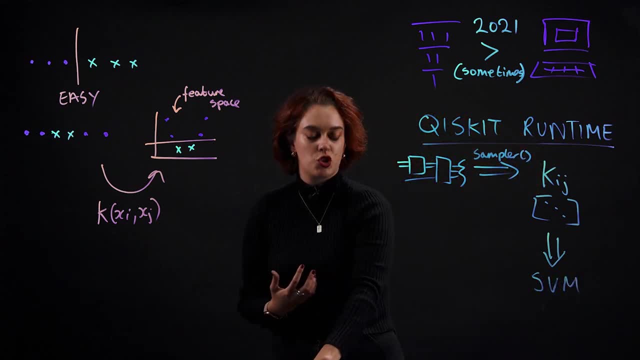 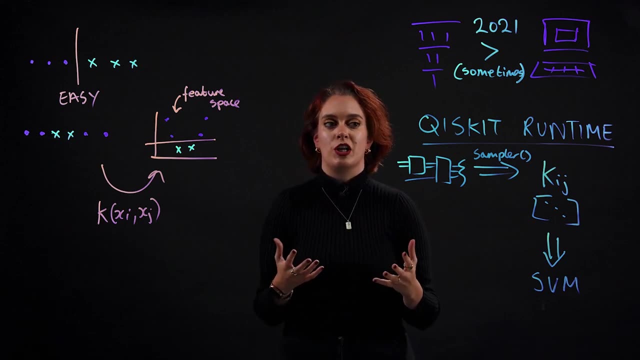 to predict new classification labels. so if you're ready to get started learning more about quantum machine learning, you can check out the links in the description for more information about qiskit runtime, as well as a quantum machine learning course that's available on the qiskit textbook. 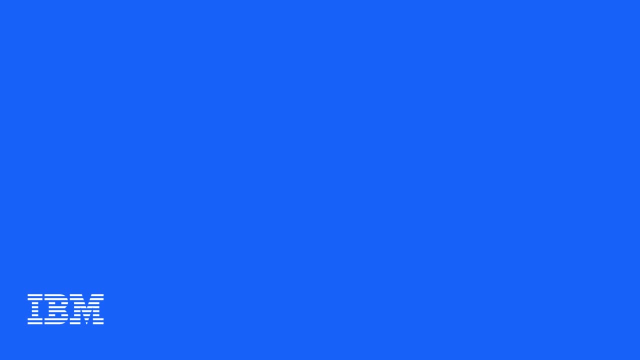 i hope you've enjoyed this video and if you have any questions, please feel free to ask them in the chat box below. thank you, hope you've enjoyed this content. thank you very much for watching.